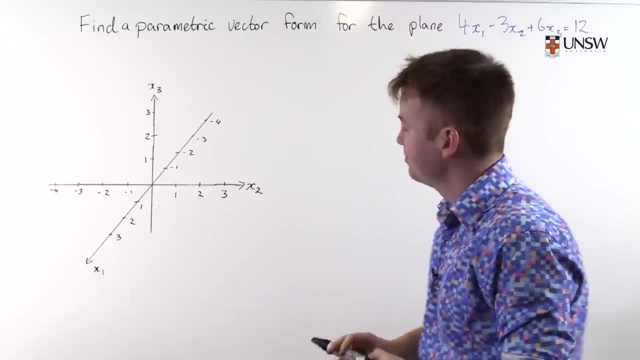 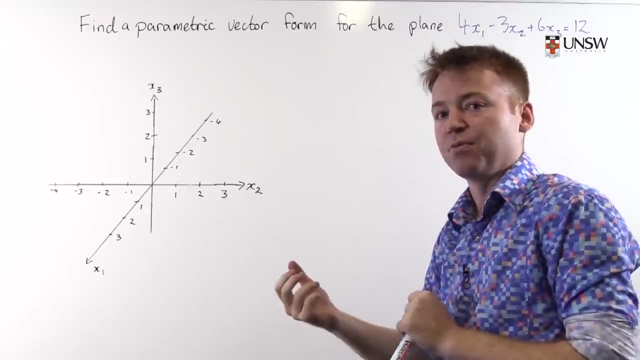 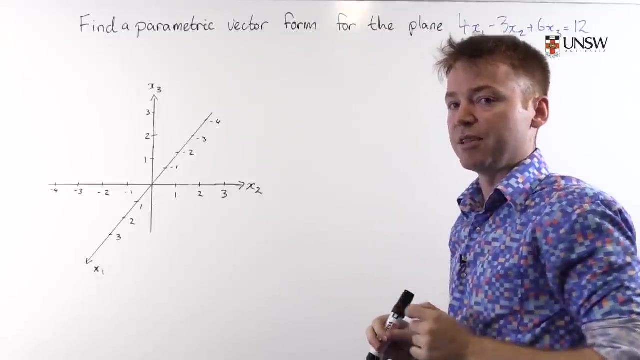 going to find one of them, and this may look different to the one that you find. We're also going to do this question in two ways. There's a first way, which is very visual, where you find some points on the plane and then from those three points, you find a parametric. 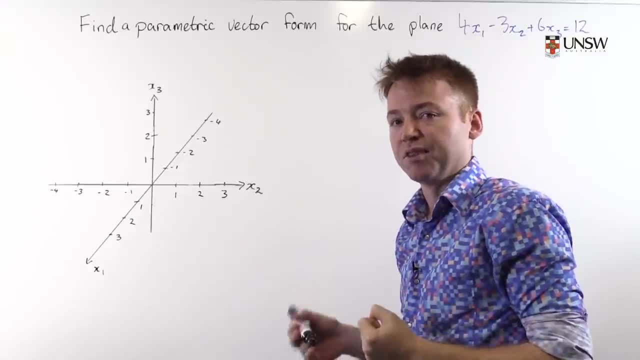 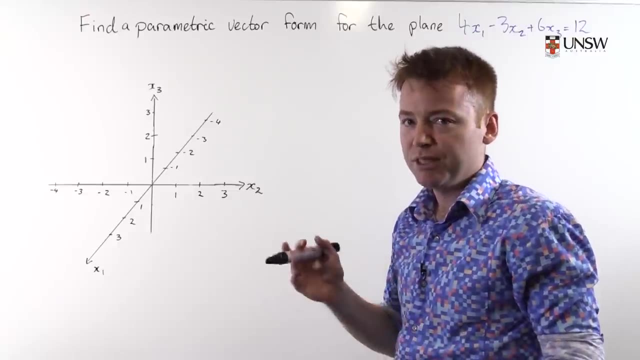 vector form of the plane, And that's nice because you get a picture and a feeling for what this plane actually looks like. There's a second way which is somewhat mechanical and straightforward and gets you the answer, but it's less visual. We will do both ways. 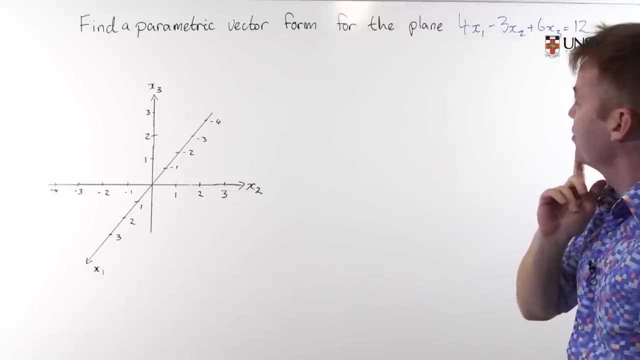 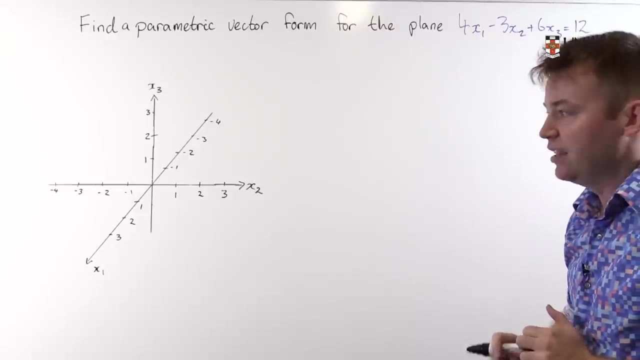 First, the visual way: Find a parametric vector form for this plane. The first way. we need three points. The easiest three points are the ones on the x1, x2 and x3 axes, So we'll find these points in much. 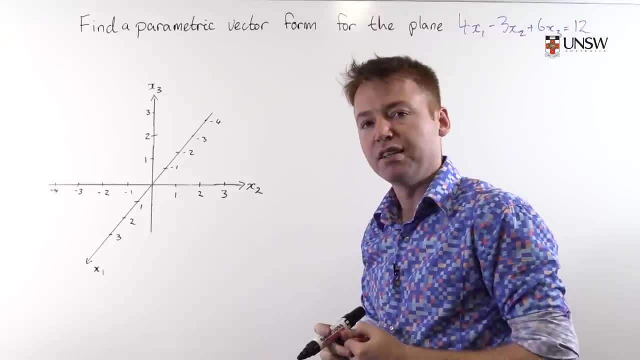 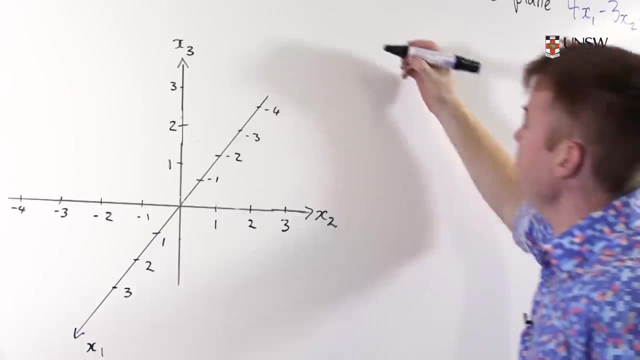 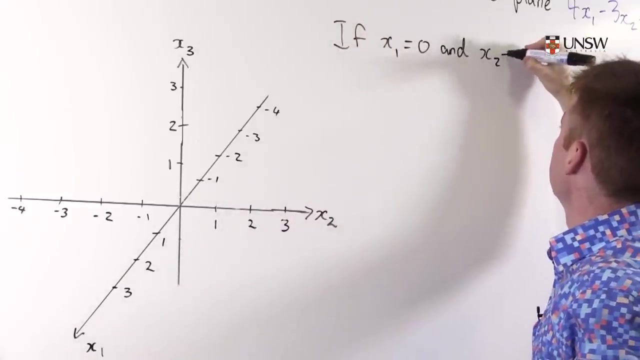 the same way as you would find them on a two-dimensional plane. in high school. We'll set, say, x1 and x2 to be equal to zero and find the x3 component If x1 is equal to zero And x2 is equal to zero. 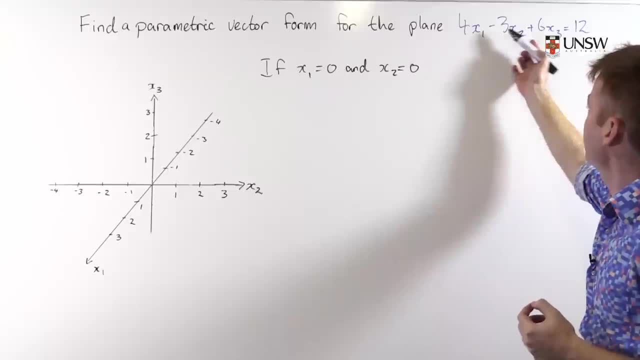 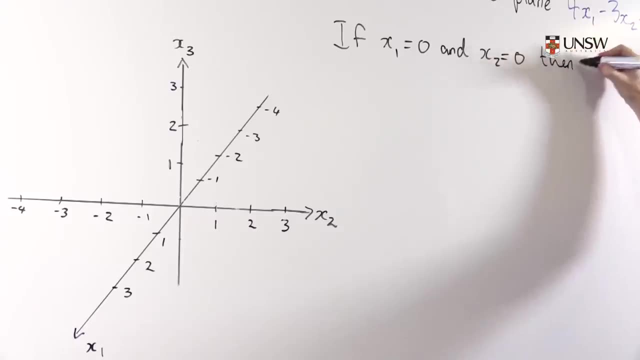 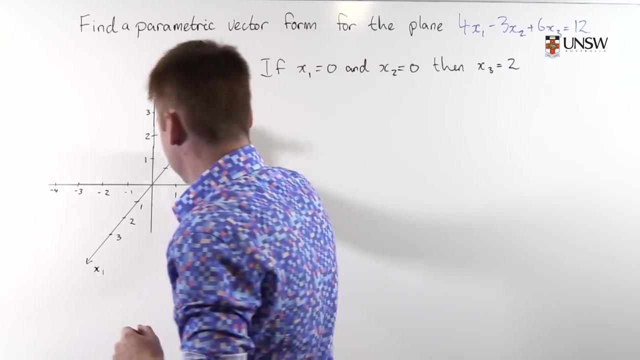 Then what must x3 be? Well, if that bit's zero and that bit's zero, then 6x3 is 12, so x3 must be 2.. Good, So, whatever this mysterious plane looks like, we know that this point we'll do it. 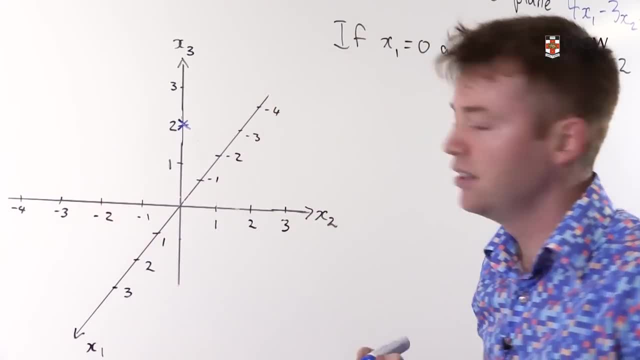 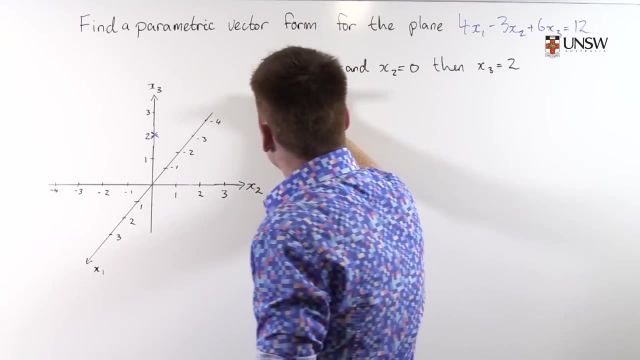 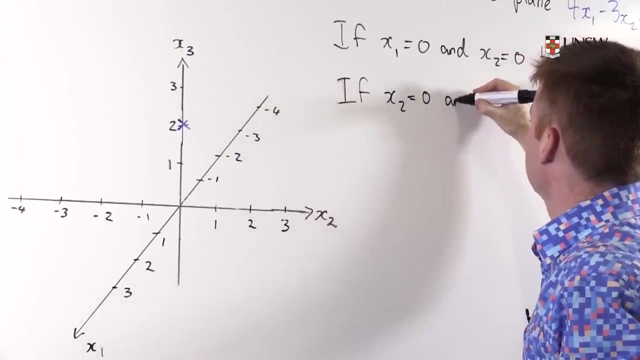 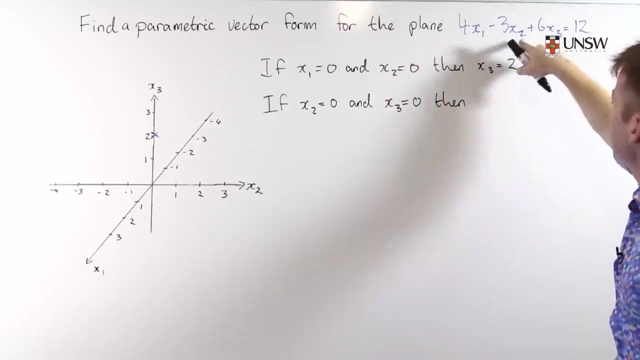 in blue. we know that this point here is on it Good, So let's carry on and find another point on this plane. If x2 is equal to zero and x3 is equal to zero, then hmm Well, if that bit's zero and 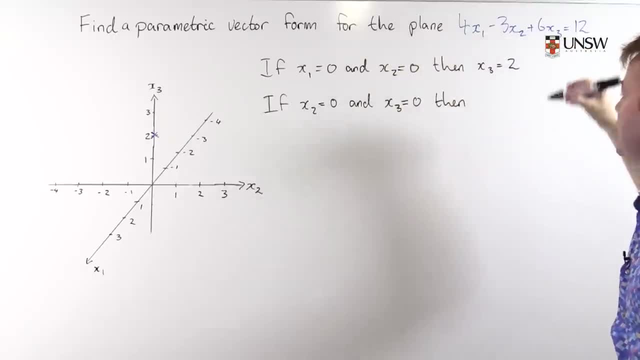 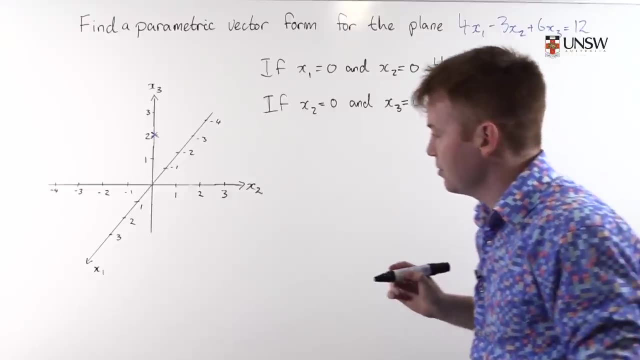 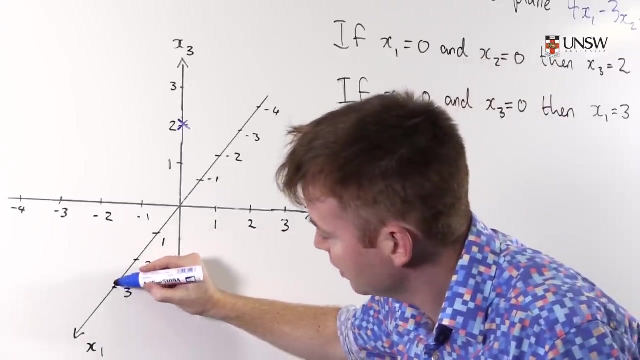 that bit's zero, then 4x1 is 12, so x1 must be 3. x1.. And we found another point on the plane with x2 and x3, zero, and in blue. here We're getting a slightly better feeling for what this plane might look like. We've got. 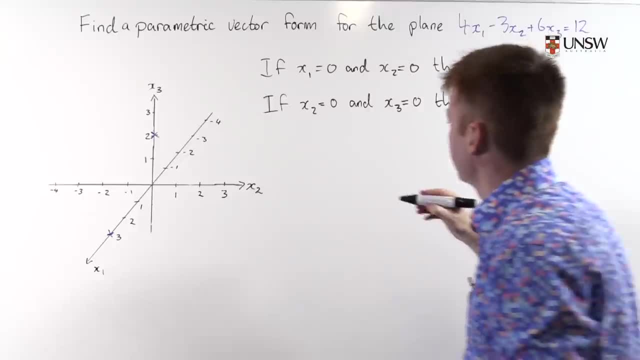 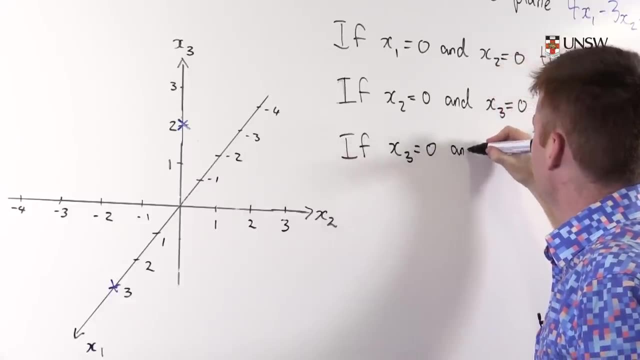 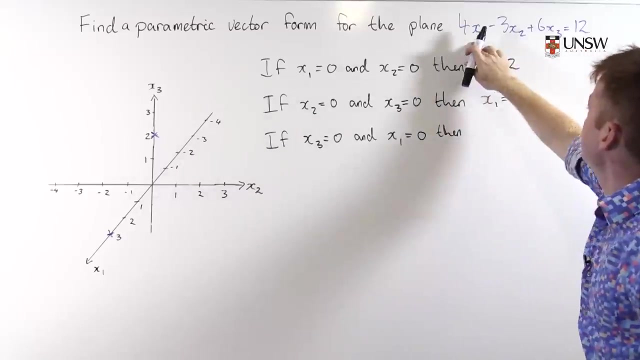 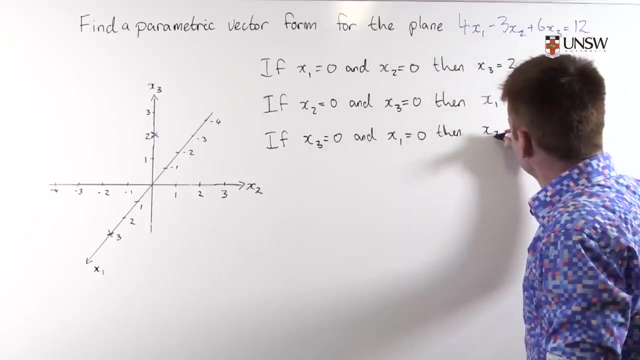 now two points on this plane. Let's find a third. If x3 is equal to zero and x1 is equal to zero, then Well, Well, if that bit's zero and that bit's zero negative, 3x2 is 12, so x2 must be equal to negative 4.. 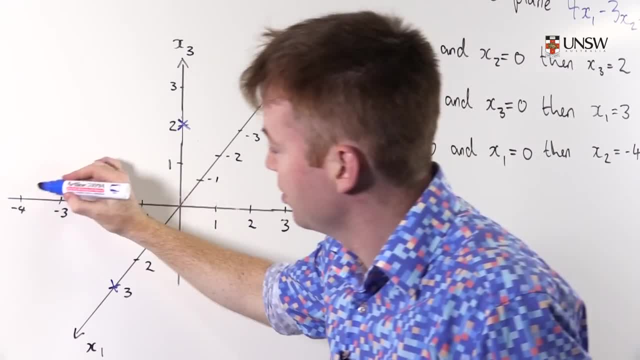 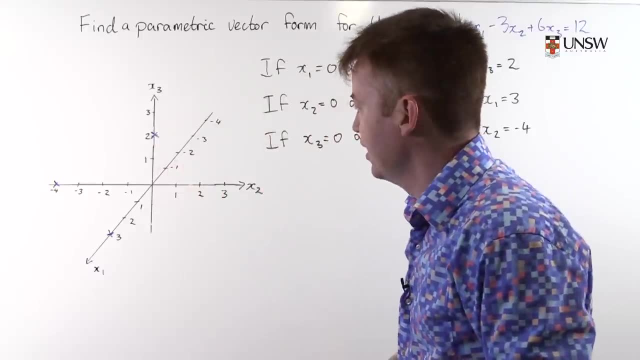 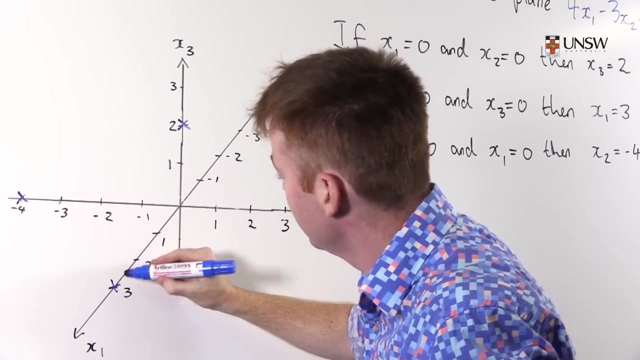 And we have our third point on the plane with x2 component negative 4, like that. Now we can actually get a feeling for what this plane looks like. It's a two-dimensional object. covering these three points Give some kind of representation. 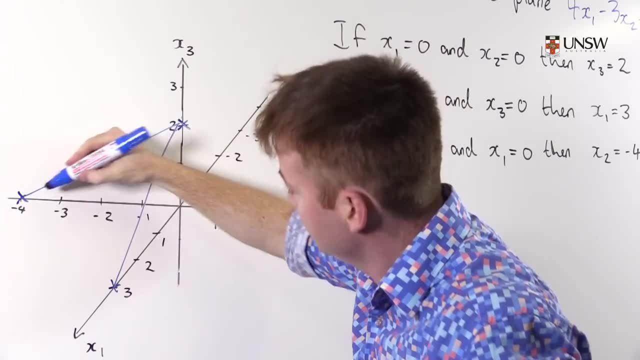 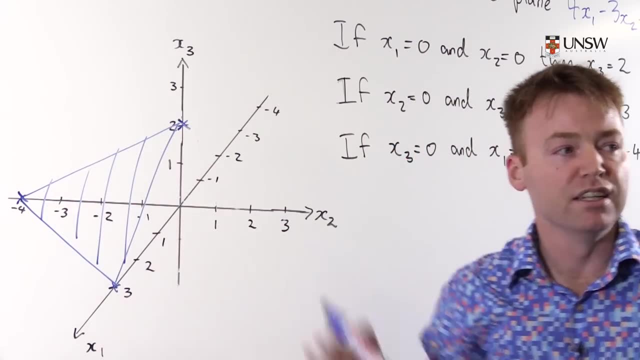 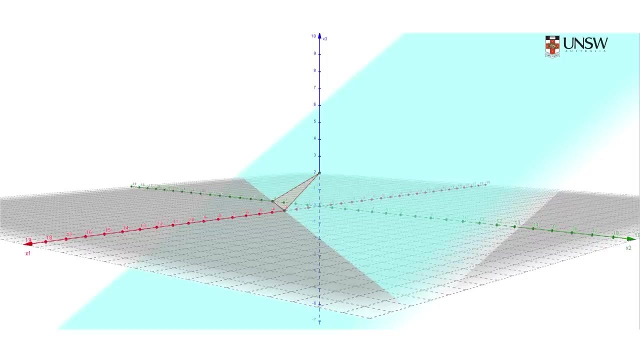 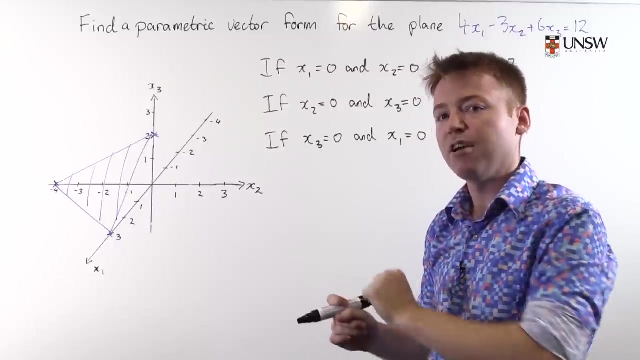 Using a triangle like this, So the cover of the surface of that triangle. And if you were to extend this triangle infinitely in all directions, then that would be a visual representation of the plane. With these three points in hand, we can find the parametric vector form of the plane. 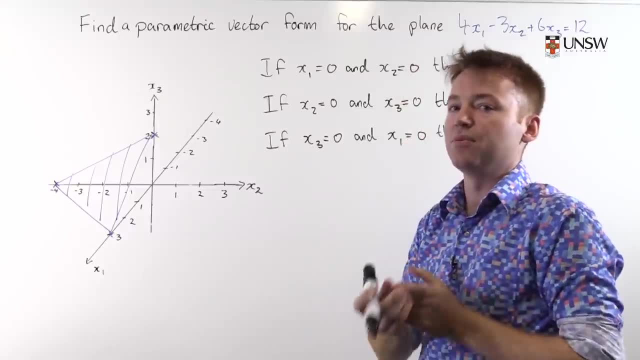 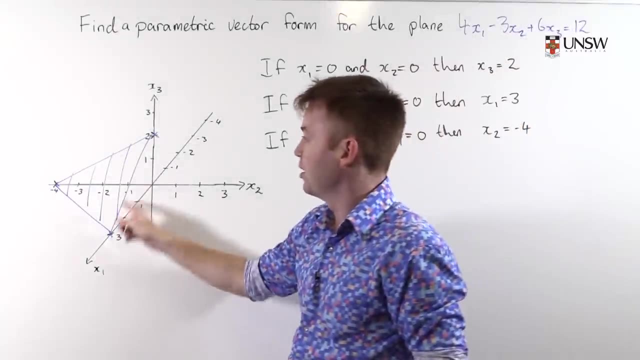 We need a point on the plane And two vectors which are parallel to the plane. This is why parametric vector form of the plane is not unique, Because it's up to you to choose one of these three points to be on the plane. 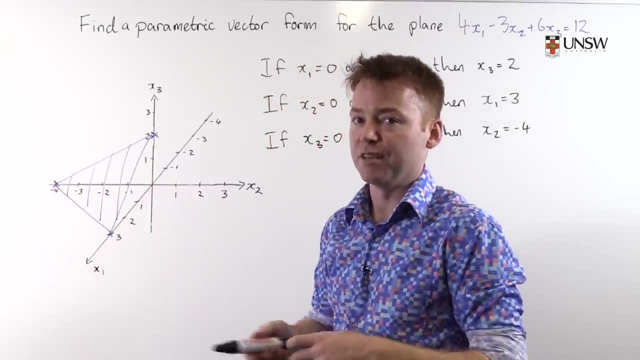 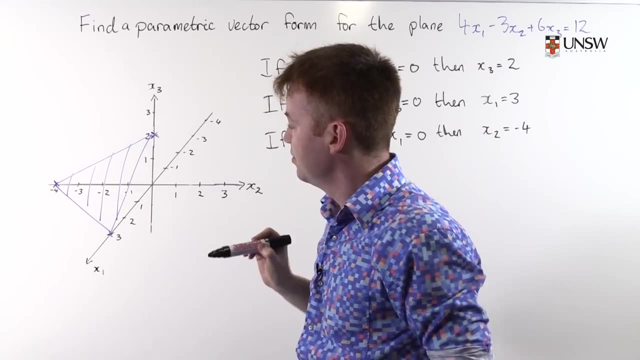 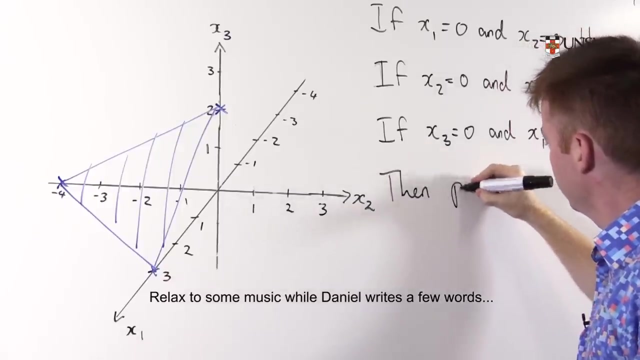 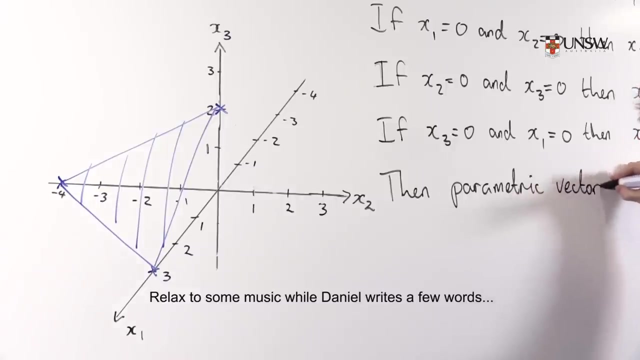 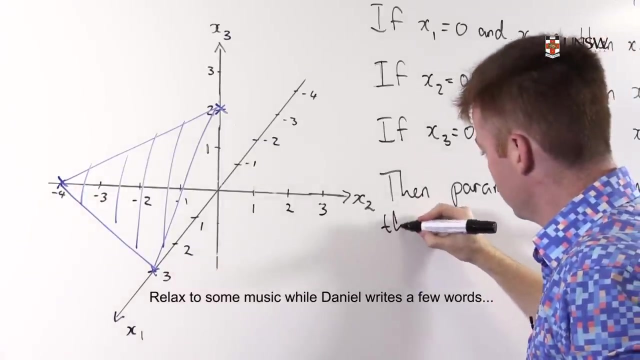 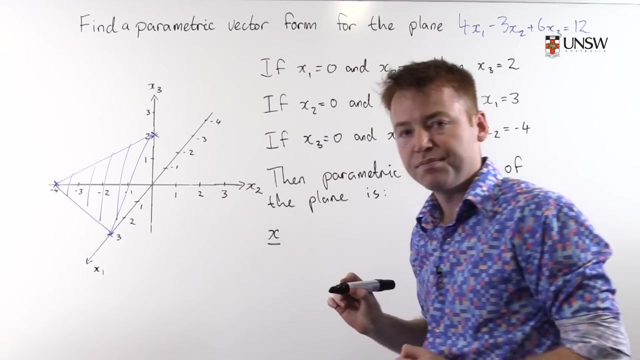 And then from there choose two vectors parallel to the plane. So there's a lot of freedom to choose your parametric vector form of the plane. Let's choose this point here to be on the plane. So x, x is equal to a point on the plane. 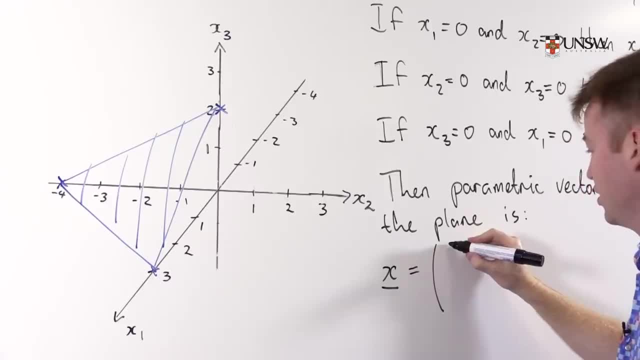 Let's choose this one With 0,, 0,, 2.. So that's x1 coordinate 0.. x2 coordinate 0.. x3 coordinate 2.. And then we need to choose two vectors that are parallel to the plane. 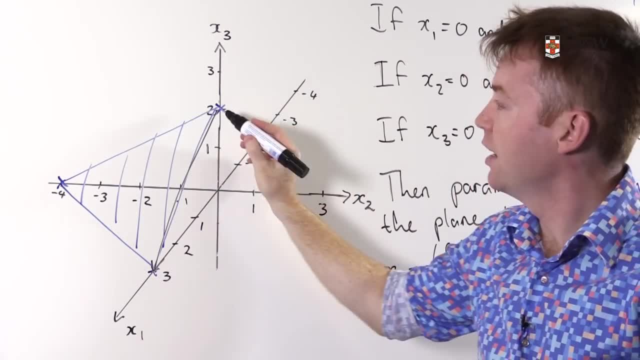 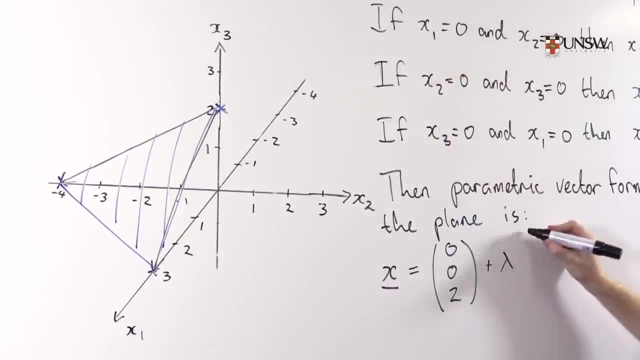 The vectors we'll choose are this vector here And this vector here. So it's lambda times. let's see Now, it's from this vector. go to this vector. So that will be 3, 0, 0.. Minus 0, 0, 2.. 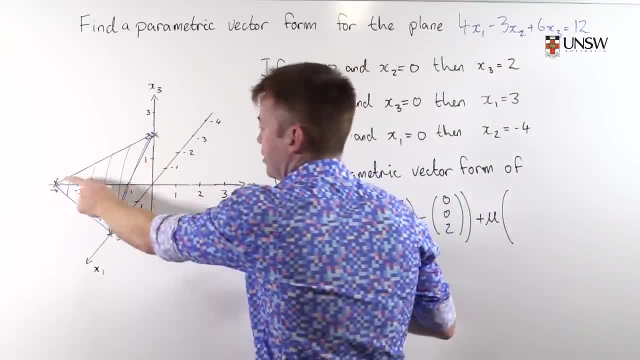 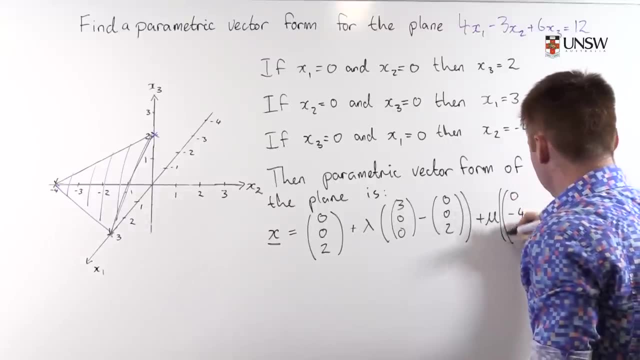 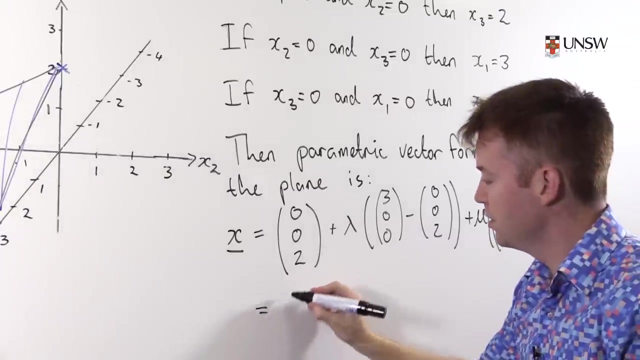 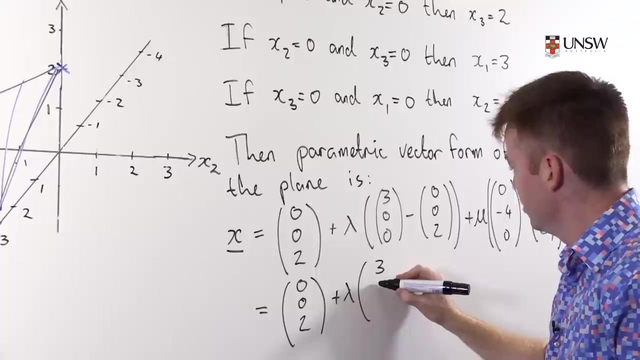 Plus mu times from this vector go to this vector: 0, negative 4, 0.. Minus 0, 0, 2. Which is 0, 0, 2.. Plus lambda times 3, 0, negative 2.. 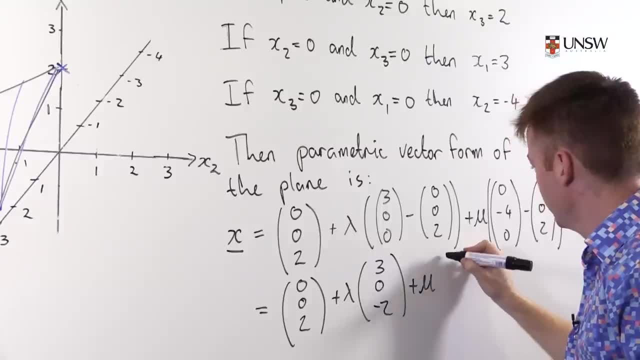 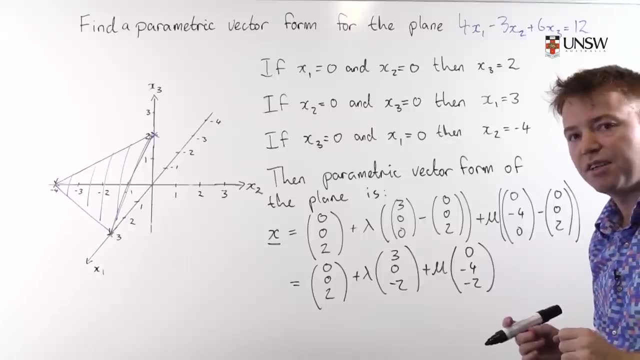 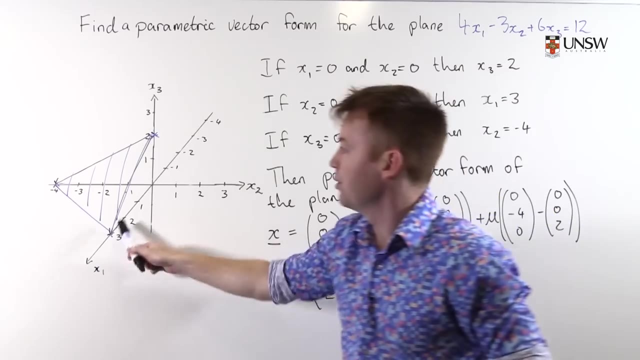 Plus mu 0, negative 4, negative 2.. And it's relatively straightforward to check that this plane, this parametric vector form of the plane, indeed does contain those points it's supposed to contain. If you set lambda to be equal, going from here, 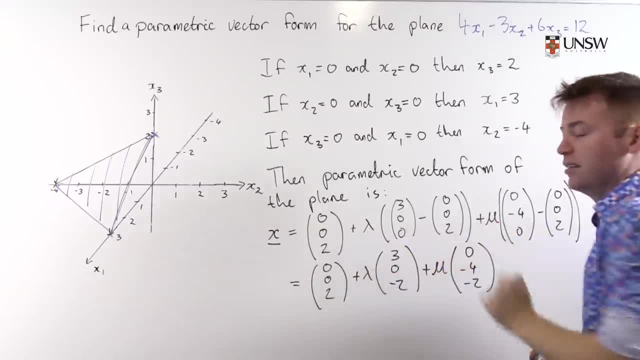 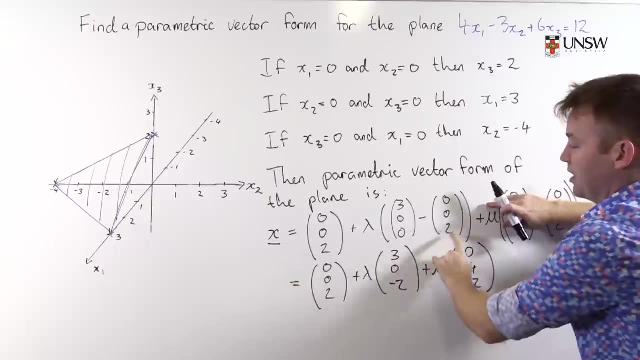 if you set lambda to be 0 and mu to be 0, then you see that this point's on the plane. If you set lambda to be 1 and mu to be 0, then you see that that bit goes away. that will cancel with that. 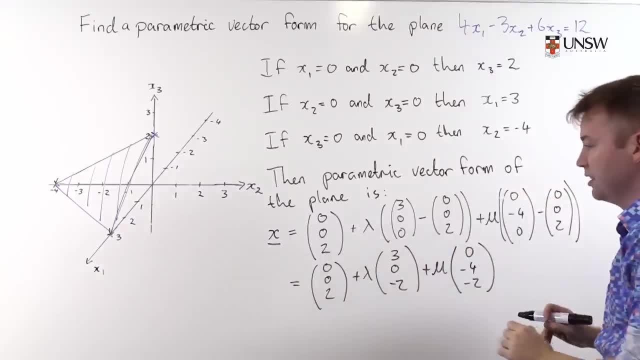 and this point's on the plane. Similarly, if you set lambda to be 0 and mu to be 1, then that goes away and this will cancel with this. so you are left with 0, negative 4, 0. 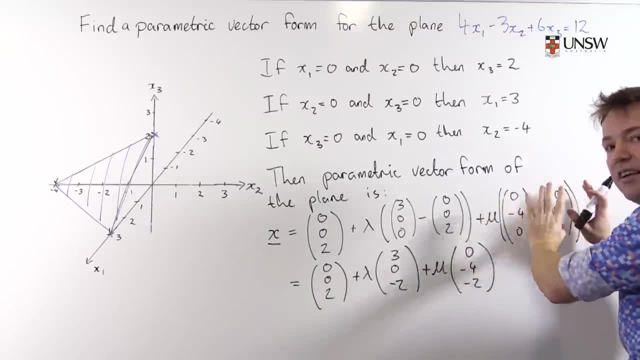 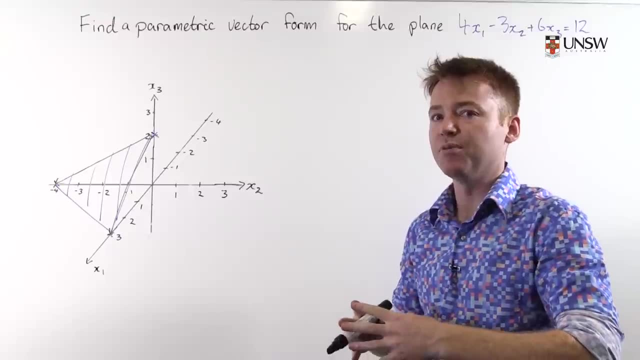 So in fact, it's easy to see just by looking at this that this is the correct. this is a correct parametric vector form of the plane. You mentioned earlier that there was a faster way of doing this question, And here it is. 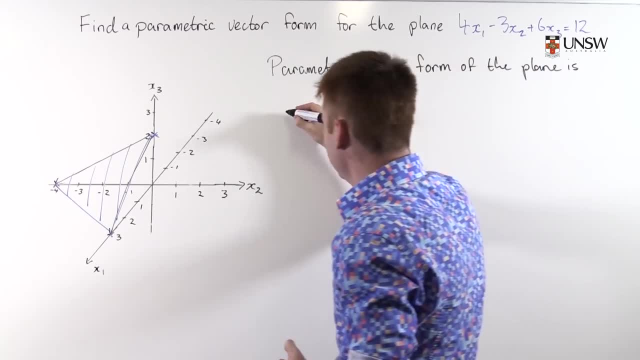 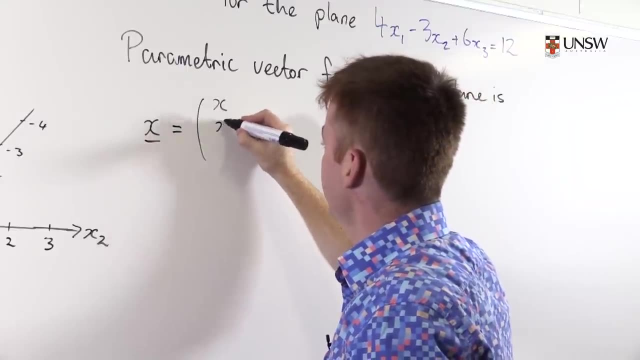 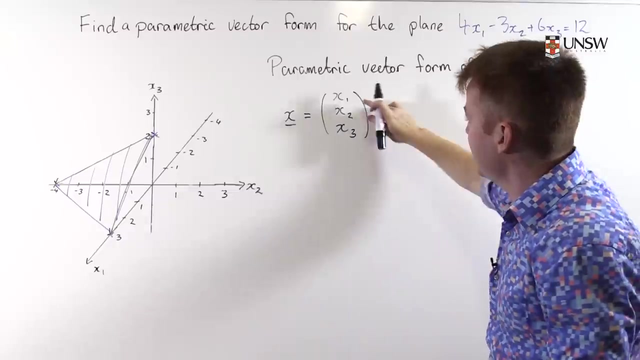 You just start writing down parametric vector form of the plane. You begin with your x vector x, like this, and you expand that a bit. you unpack your x with x1, x2, x3, like that, And then you replace one of these symbols. 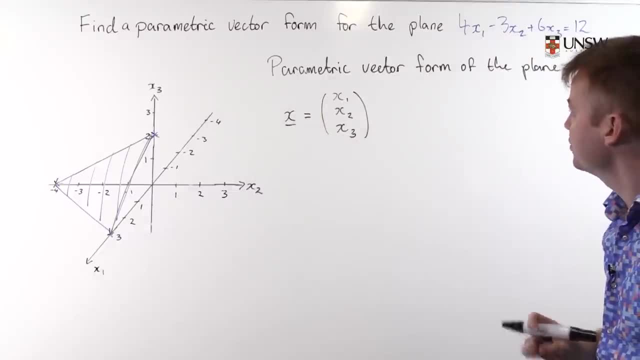 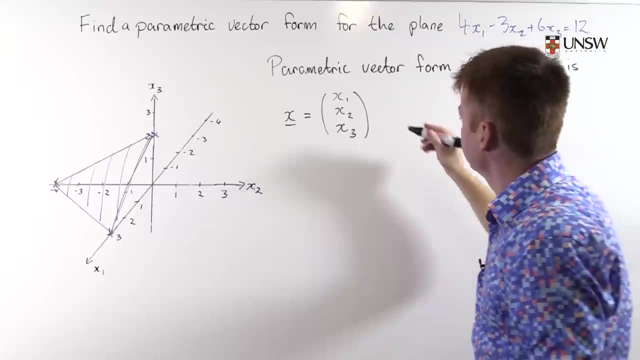 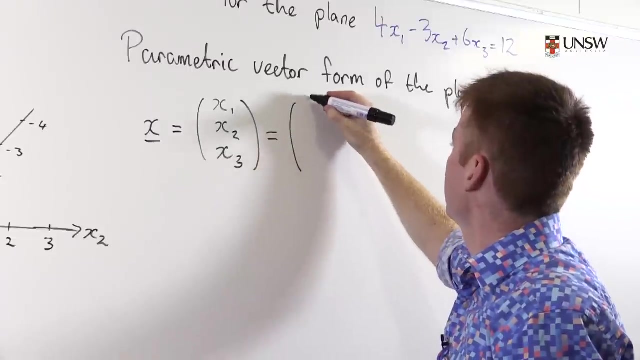 with one of those symbols from Cartesian form of the plane. You may not have all the symbols available to you, but you have to choose one. I'm going to select x1. And I will replace x1 with its expression up here. So that's 1 quarter of 12,.